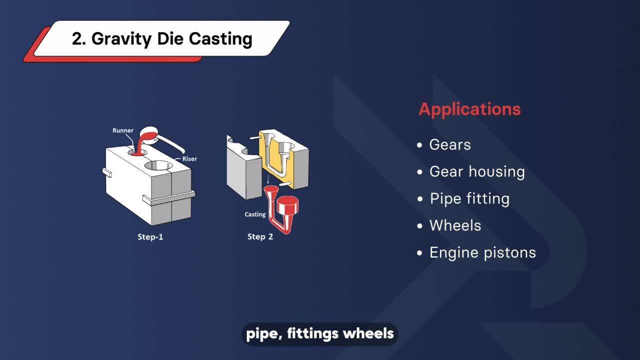 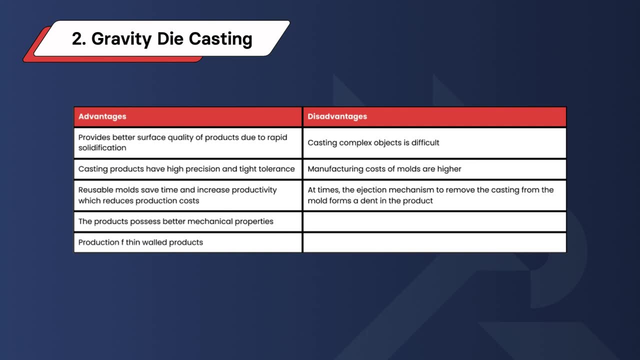 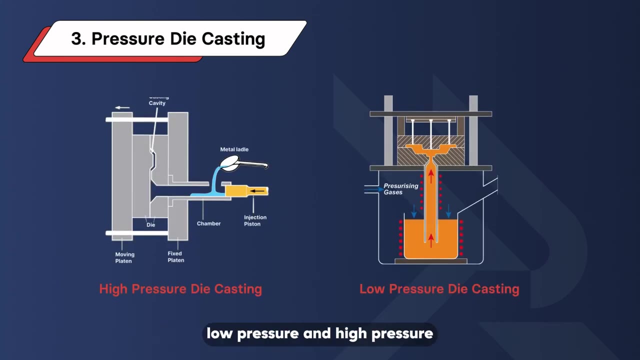 parts like gears, gear housing, pipe fittings, wheels, engine pistons, etc. Advantages and disadvantages: Pressure- die casting. Pressure die casting comes in two varieties: low pressure and high pressure. High pressure die casting is ideal for mass-producing. 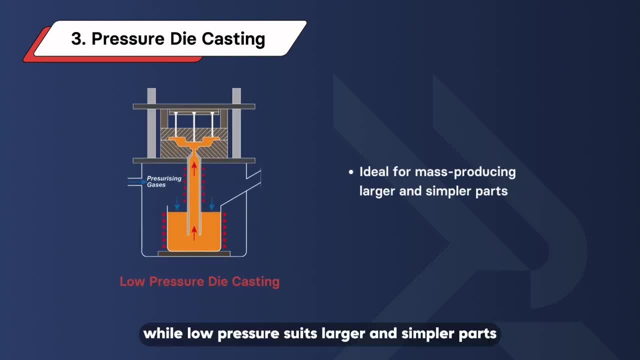 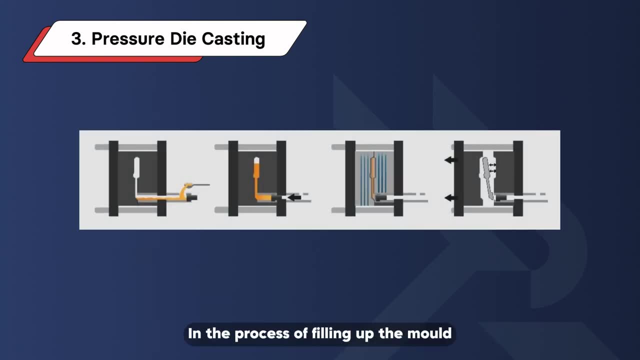 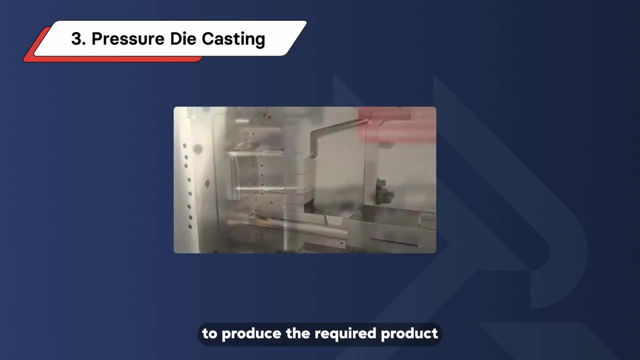 intricate, precise components, while low pressure suits larger and simpler parts. Pressure die casting differs from gravity die casting in the process of filling up the mold. where pressure die casting uses high-pressure injection of molten metal into the metal mold. The molten metal is then solidified rapidly to produce the required product. 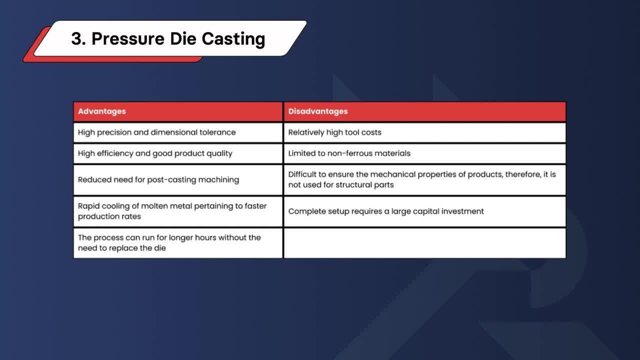 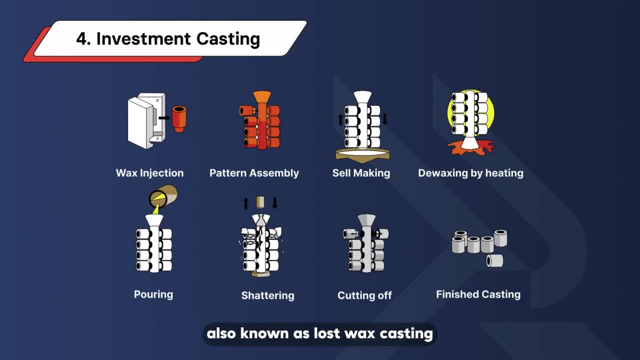 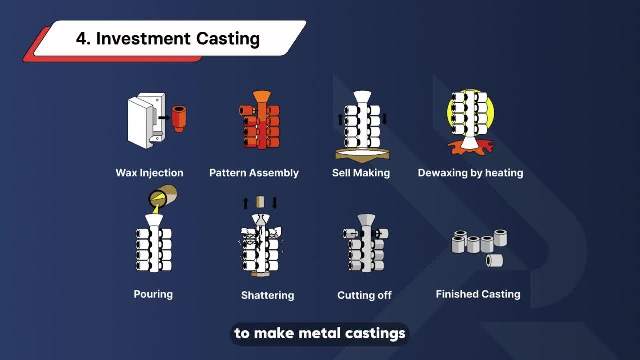 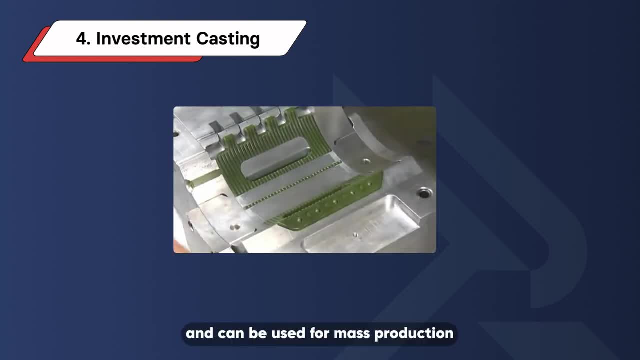 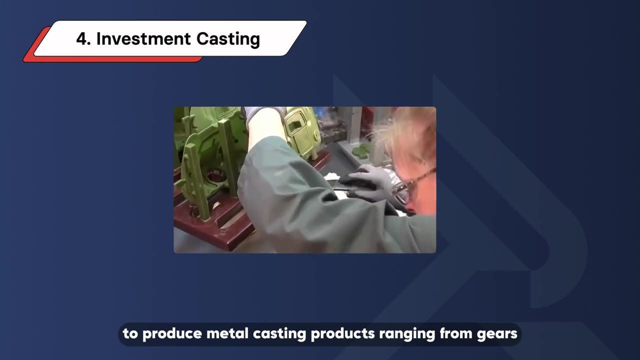 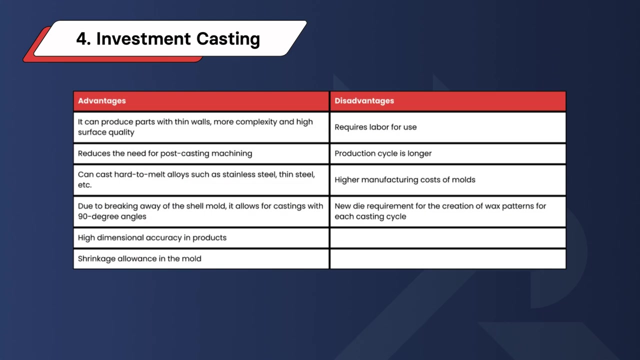 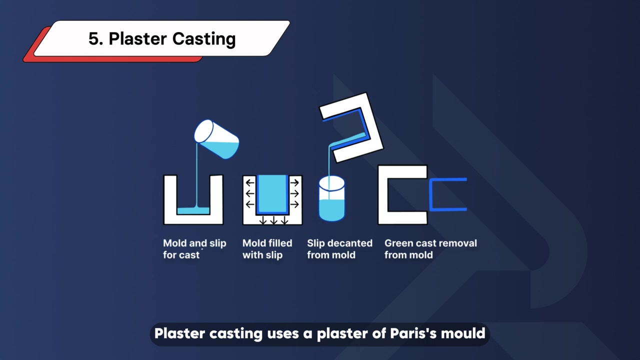 molten metal is poured into the mold to make metal castings. Investment casting is an expensive and labor-intensive process and can be used for mass production or in complex casting. Our most advanced master builders in the Early Gamers discussed and reviewed this in depth. 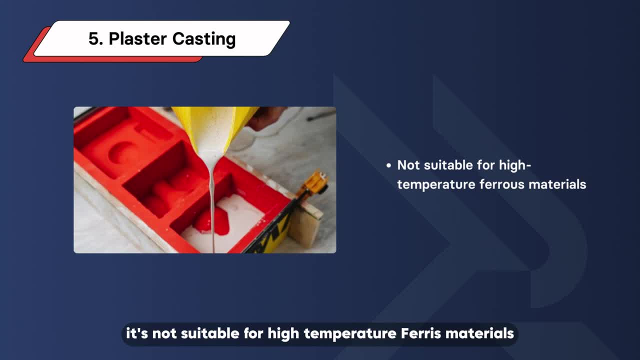 Advantages and Disadvantages. Plaster Casting. Plaster casting uses a plaster of persön Ray Fl raising mold which cools the metal more slowly, allowing for high-accuracy, especially with thin cross-section parts. However, it's not suitable for high temperature ferrous materials. 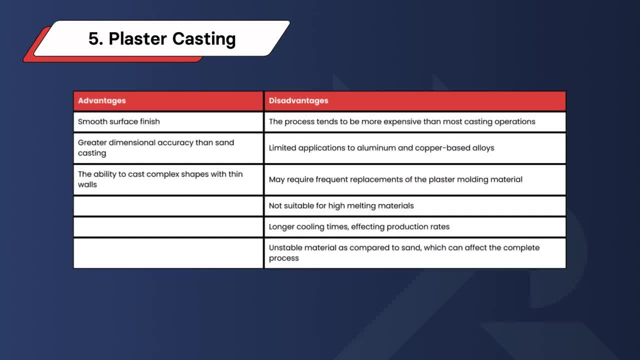 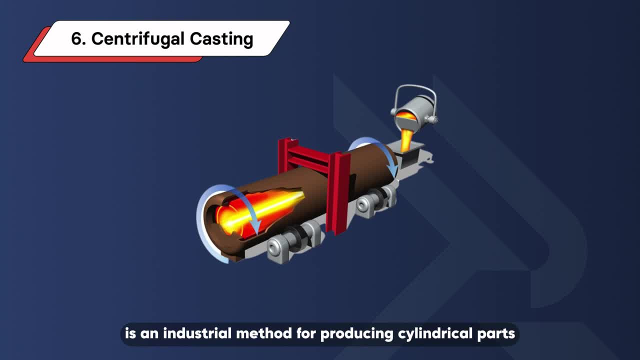 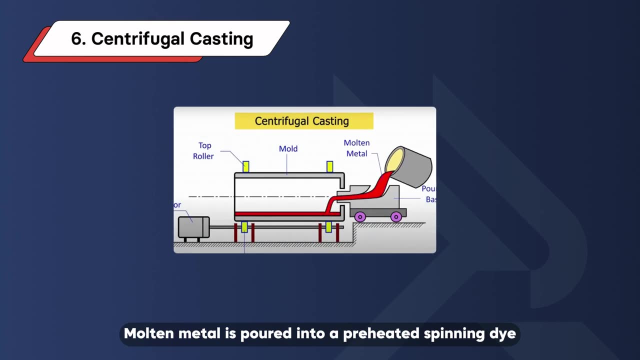 Advantages and disadvantages and disadvantages: Centrifugal casting. Centrifugal casting or rotocasting is an industrial method for producing cylindrical parts using centrifugal forces. Molten metal is poured into a preheated spinning die and the centrifugal forces distribute the metal within the die. 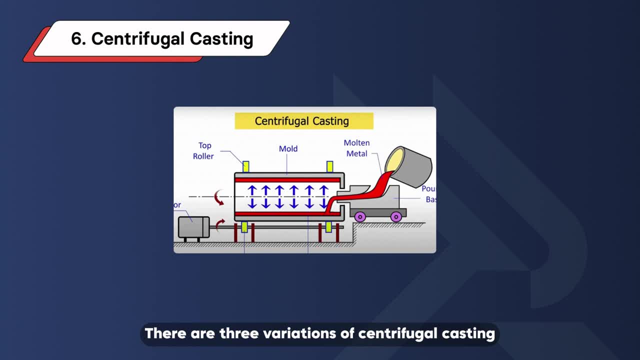 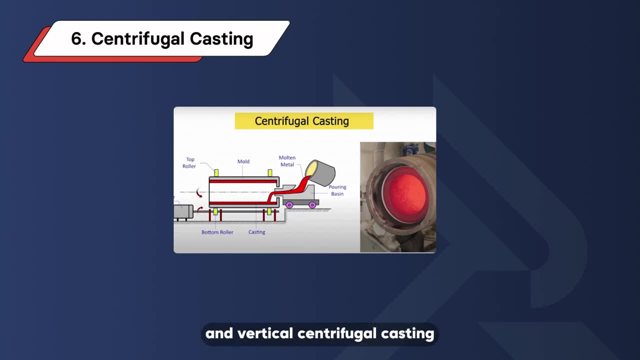 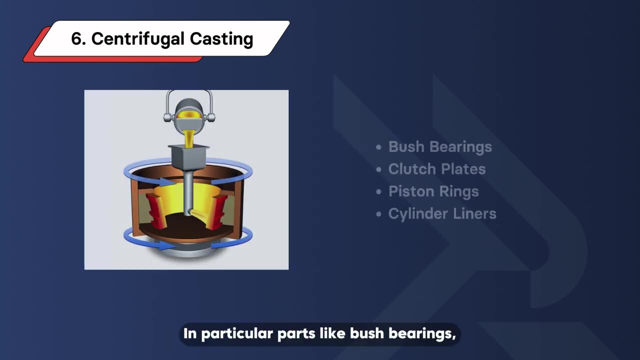 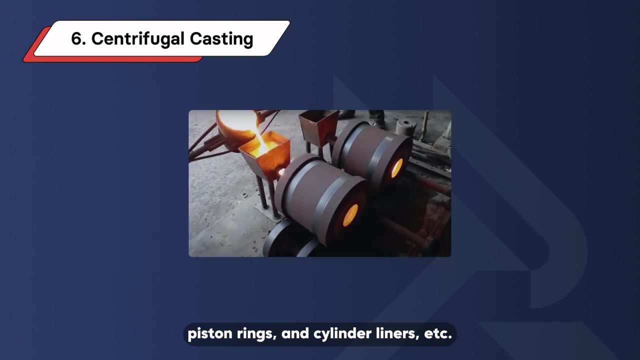 under high pressure. There are three variations of centrifugal casting: True centrifugal casting, semi-centrifugal casting and vertical centrifugal casting. Typically, centrifugal casting produces rotational shapes like cylinders, In particular parts like bush bearings, clutch plates, piston rings and cylinder liners, etc. Also the pouring of metal in the center of 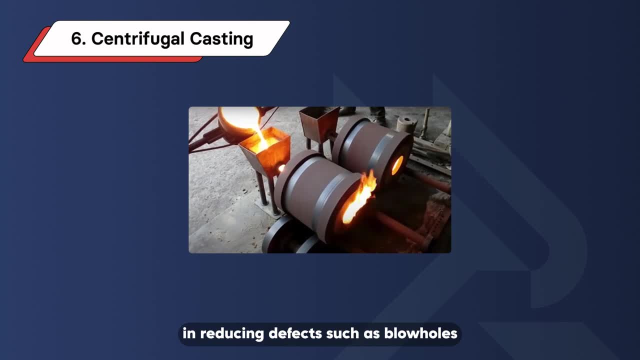 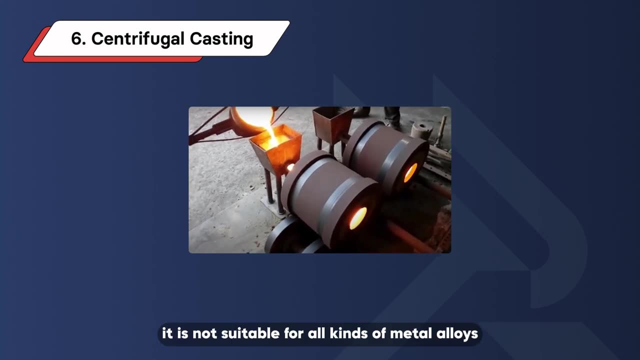 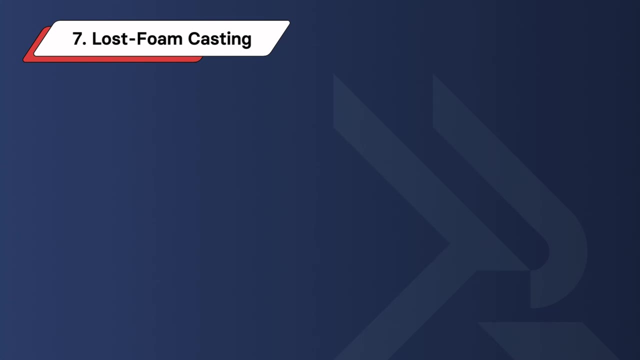 the mold helps in reducing defects such as blow holes, shrinkage and gas pockets. However, it is not suitable for all kinds of metal alloys. Advantages and Disadvantages. Lost foam Casting. Lost foam casting is similar to investment casting, but uses foam for the pattern. 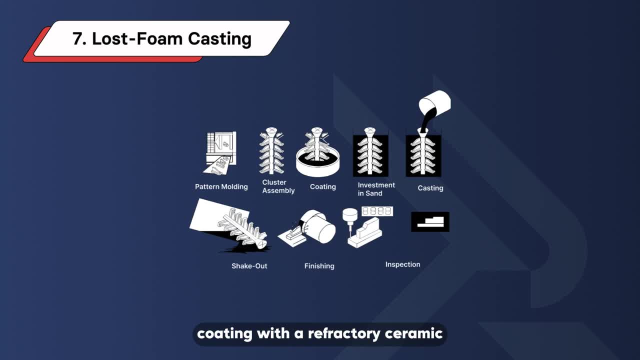 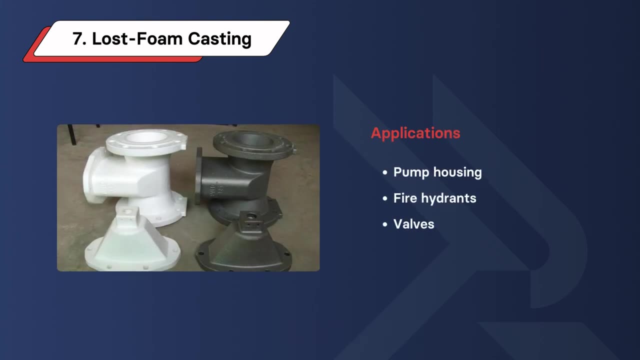 Once the pattern is formed, coating with a refractory ceramic takes place by dipping, coating, spraying or brushing. Then the molten metal is poured into the mold to form the desired product. It's suitable for materials like alloy steel and carbon steel making products like pump housing, fire hydrants and valves. 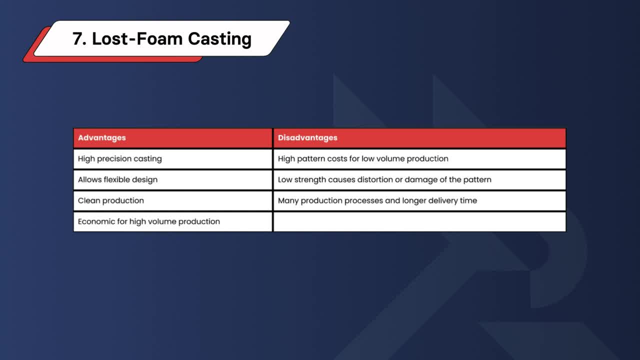 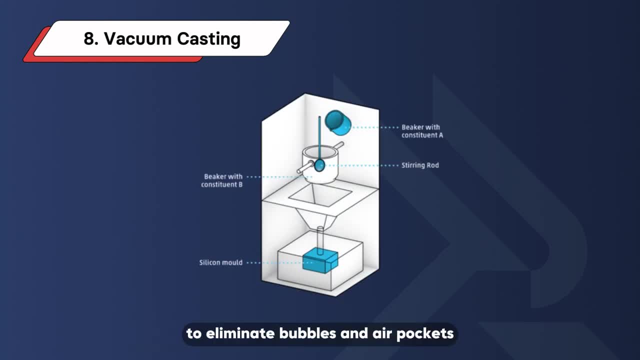 Advantages and Disadvantages: Vacuum Casting. Vacuum casting takes place under vacuum pressure to eliminate bubbles and air pockets. It's used for components like structural chassis components and automotive body parts. Advantages and Disadvantages: Squeezing Casting. 3. Squeezing Casting. 4. Squeezing Casting, 5. Squeezing Casting, 6. Squeezing Casting, 7. Squeezing Casting, 8. Squeezing Casting, 9. Squeezing Casting, 10. Squeezing Casting. 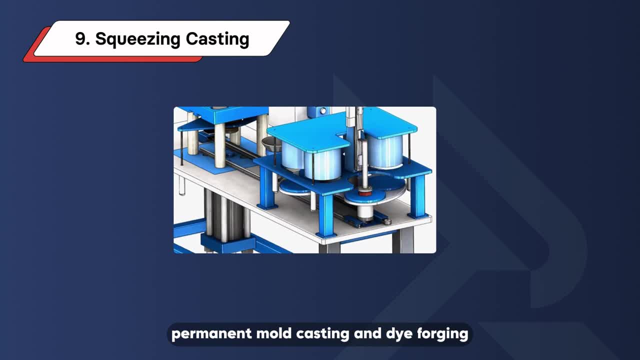 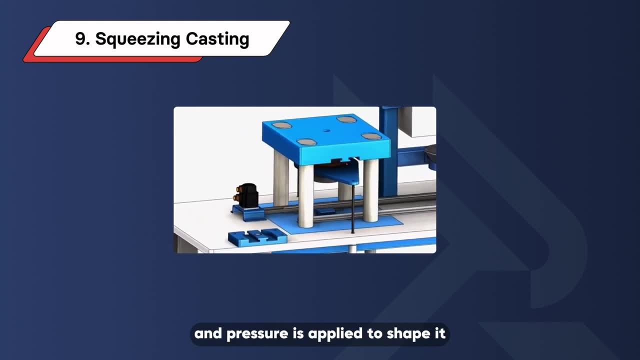 60. Squeezing Casting: hybrid process that merges permanent mold casting and dye forging. In this process, a specific amount of molten metal alloy is injected into a dye and pressure is applied to shape it. Then the metal part is heated over melting temperature and extracted from the dye. 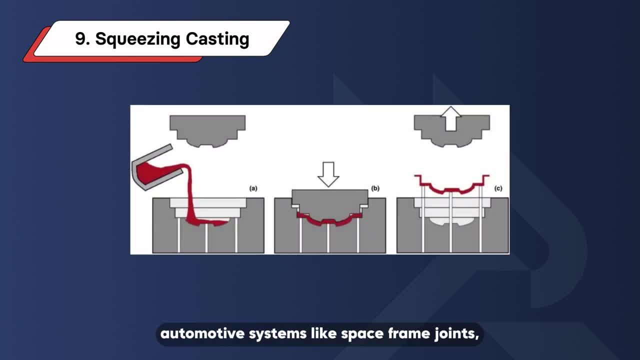 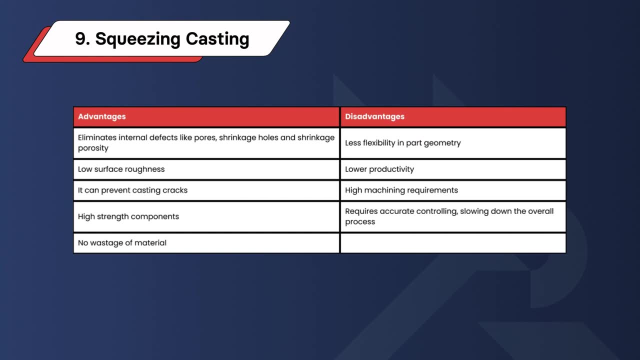 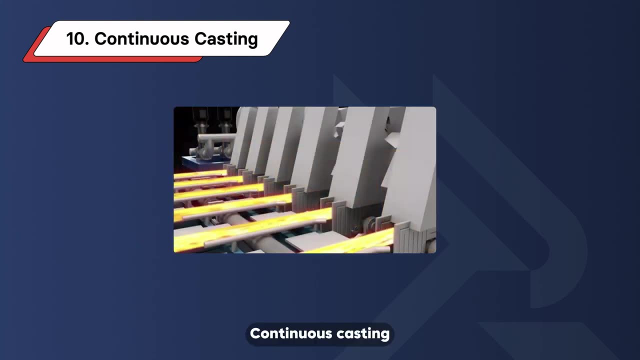 It's ideal for producing safety-critical parts in automotive systems like space frame joints, aluminum front, steering knuckles and more. Advantages and Disadvantages: Continuous Casting: Continuous casting allows consistent mass production of metal profiles with a constant cross-section, making it popular in the production.